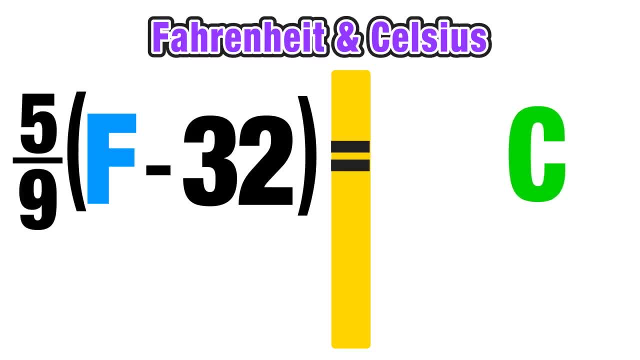 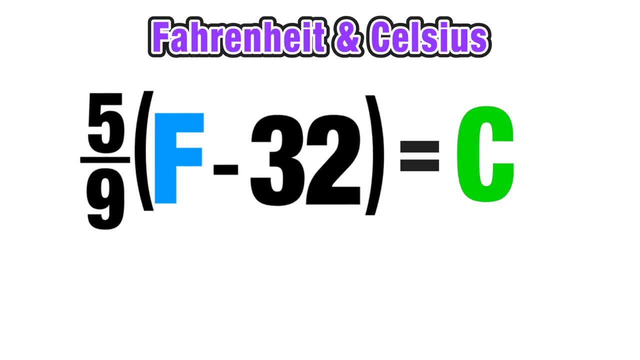 9. On the right side, those fractions will cancel out. Now we have C by itself and we see here. now we have the formula for converting degrees Fahrenheit to degrees Celsius. Now we're ready to go ahead and familiarize ourselves with using these formulas to convert back. 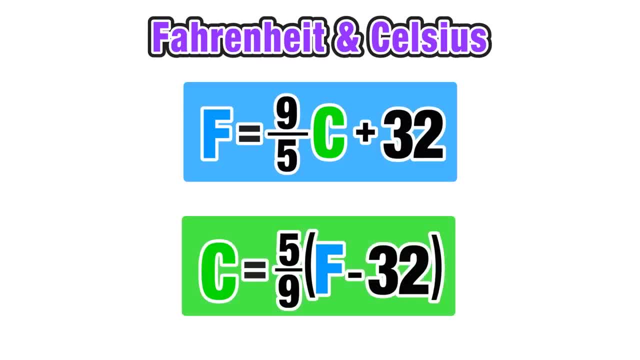 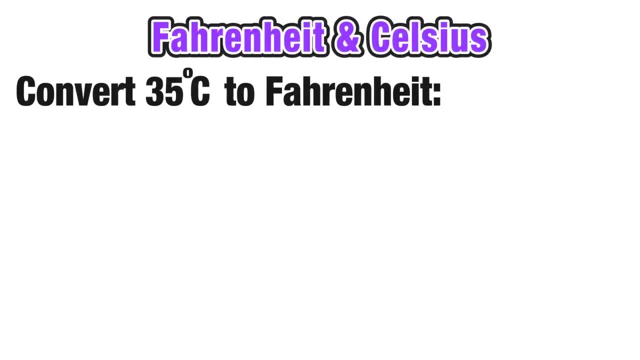 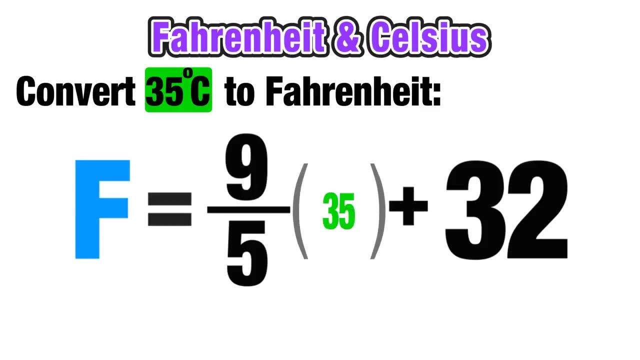 and forth between degrees Fahrenheit and degrees Celsius. So for our first example, we want to go ahead and convert 35 degrees Celsius to degrees Fahrenheit, So we want to use the Fahrenheit formula here, So we can substitute 35 for C, and now all we have to do is evaluate. 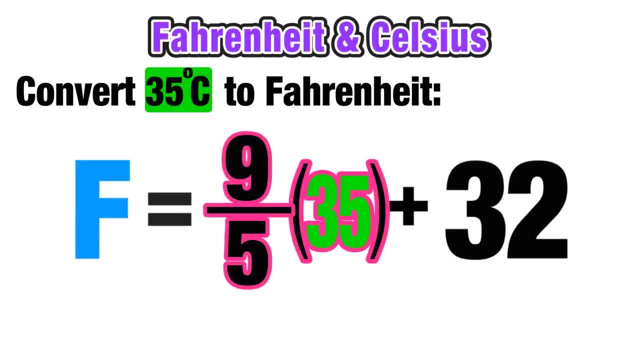 9 over 5 times 35, so we get 12 degrees C. So we can substitute 35 for C. and now all we have to do is evaluate 9 over 5 times 35, and now all we have to do is do the same. 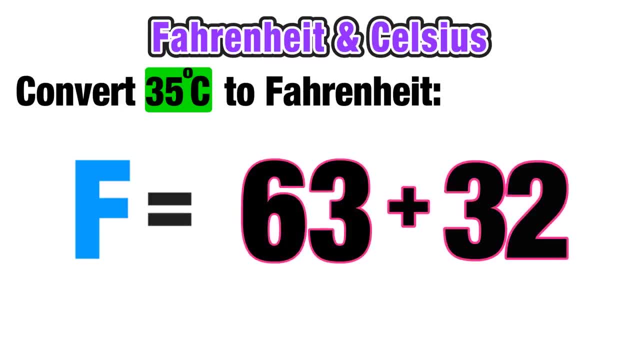 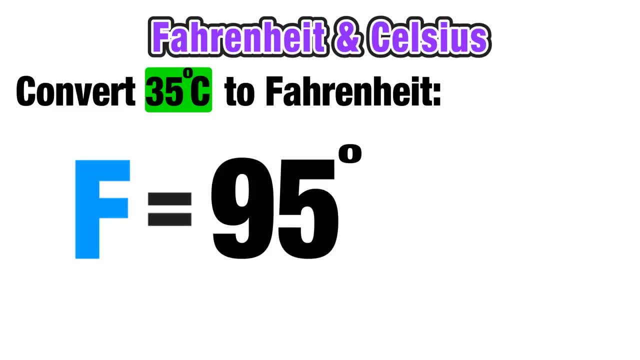 is equal to 63, and then 63 plus 32 equals 95, the number of degrees in Fahrenheit. So if you're used to the Fahrenheit scale, if you saw 35 degrees, you might think that that represents a very cold temperature, but in reality in 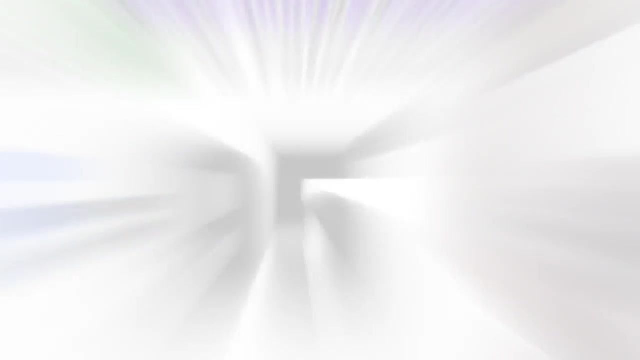 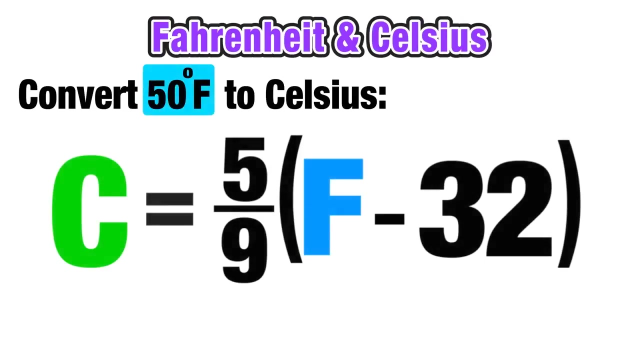 degrees Fahrenheit, it is a very warm temperature. Now for our next example. we want to convert 50 degrees Fahrenheit to degrees Celsius, so we're going to use the Celsius formula here. start by replacing F with 50 and now just evaluate: 50 minus 32- in parentheses- is equal to 18, and then 5 over 9 times 18. 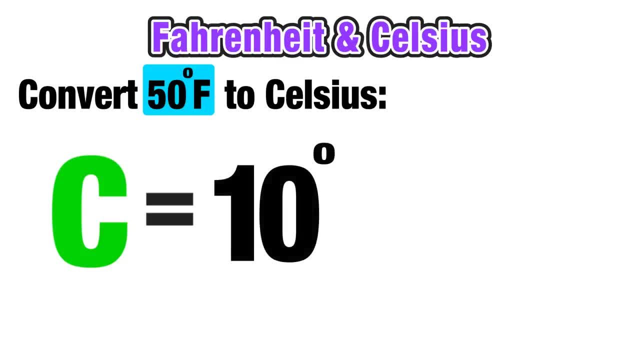 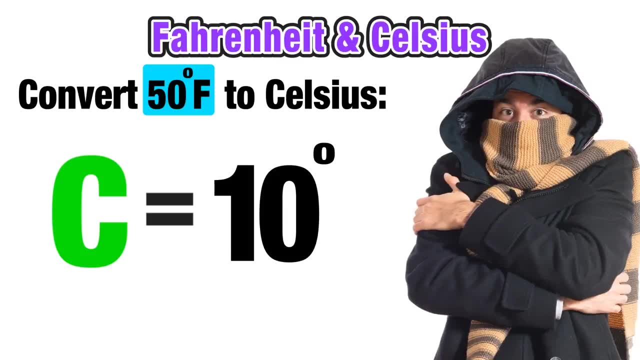 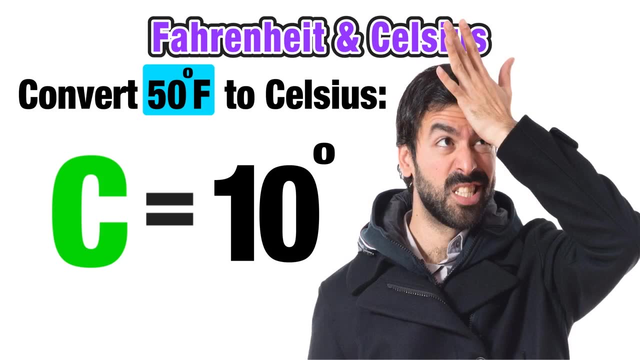 is equal to 10.. So again, if you're used to degrees Fahrenheit, if you saw 10 degrees, you might think that the weather is going to be pretty cold, when actually it's really not even that bad. Thank you again, everyone, for joining us and please reach out to us on Twitter at. 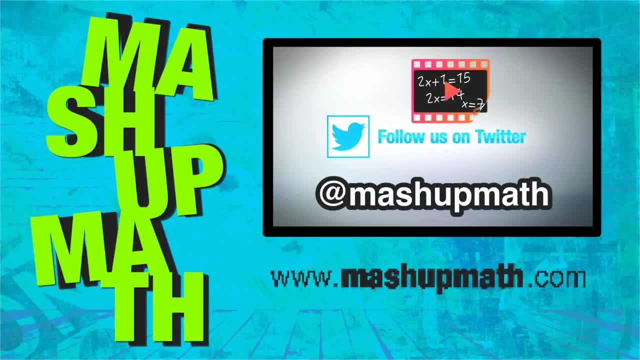 MashupMath, We are dying to hear from you, so please share some love. Alright, we're done here.